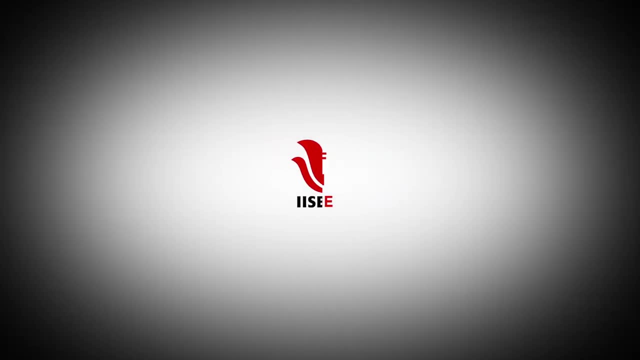 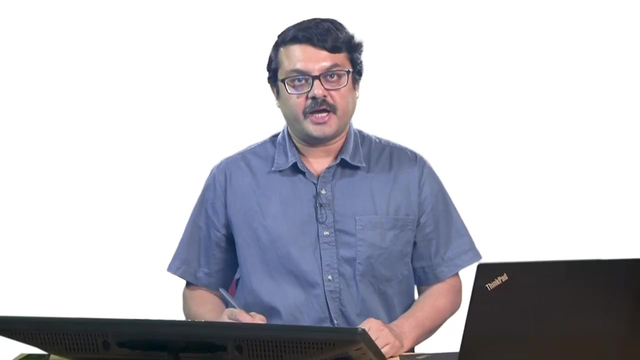 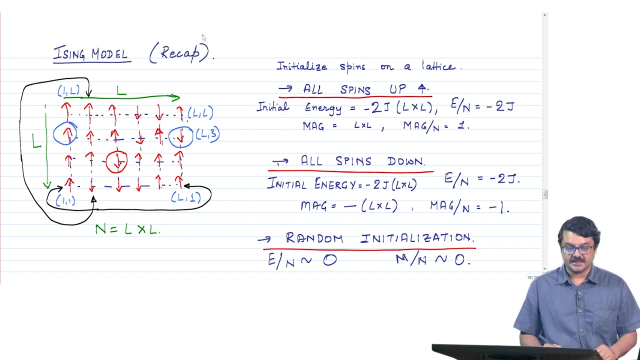 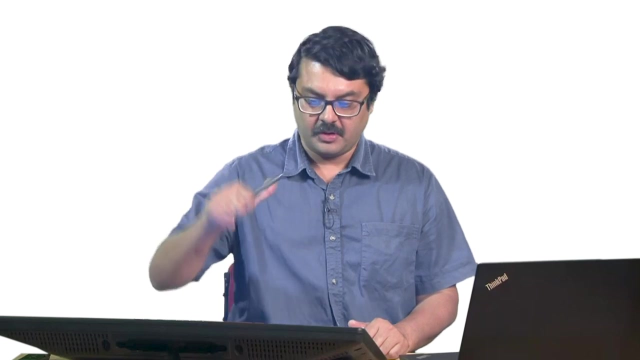 Welcome back. What I am going to start with today is having a quick recap of what we discussed in the last classes. We were discussing Ising model, in which there are spins on a lattice which can either point up or down with the which are interacting with. any spin is interacting. 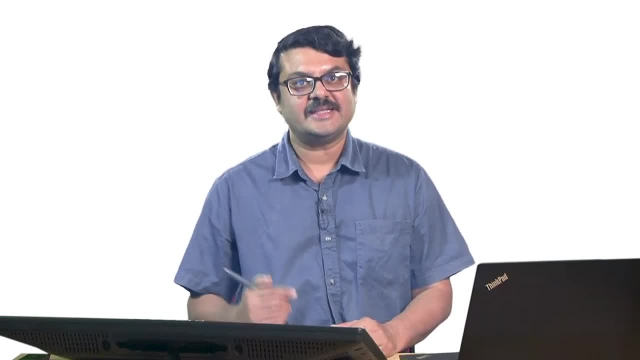 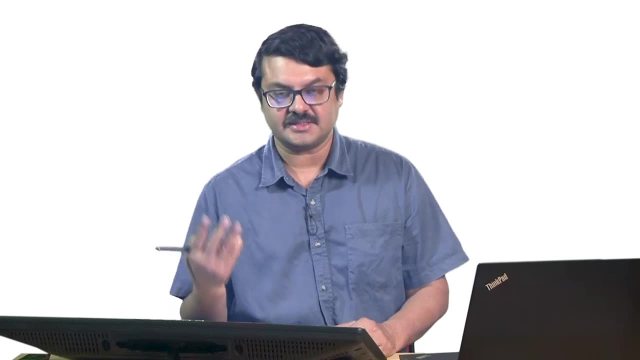 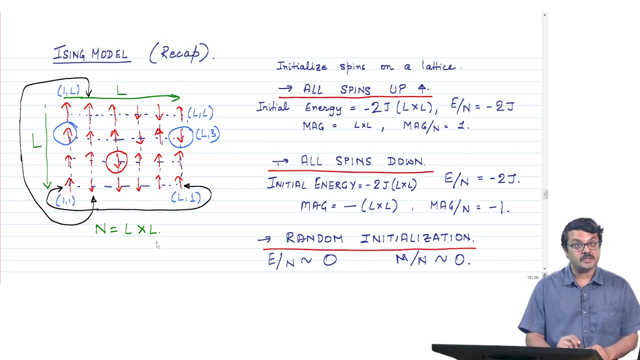 with its neighbors. with the Ising Hamiltonian, which is minus j sum, over si dot sj, where any spin interacts with its nearest neighbors, which in a 2D case is just its 4 nearest neighbors, The size of the lattice was given by L, and then the total number of spins is L cross. 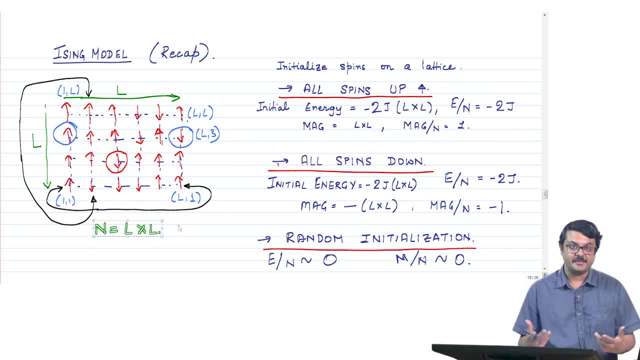 L in a 2-dimensional lattice. If you have a 3-dimensional lattice, then the total number of spins will be L cross L cross L. In the last class we discussed about initializing the spin on the lattice, So you can initialize the spins where all the spins are basically. 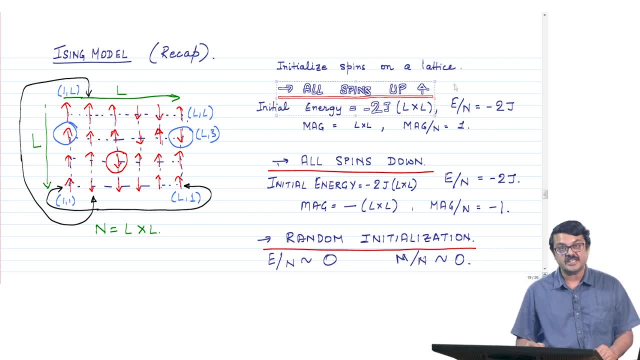 pointing up In that case that the initial energy of the energy. So all this right even before starting the Monte Carlo iterations simulations, you are going to basically initialize all the spins. you can do it as up or down, or even you could have a random initial condition. If you have a, if you start with all the spins. 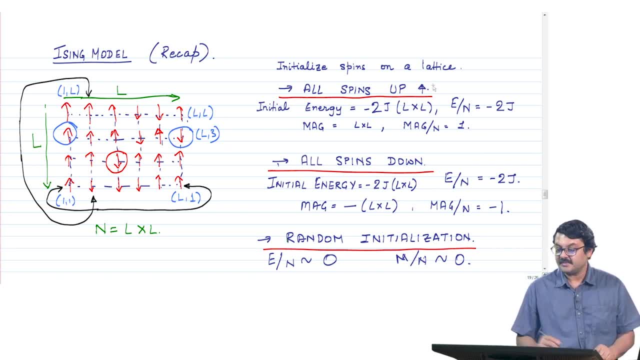 up. then the total initial energy of the system will be minus 2 j. L cross L. right, L cross L being the number of spins in the lattice, The energy per spin will be minus 2 j right. The magnetization will be L cross L and magnetization per spin will be plus 1, because all the spins 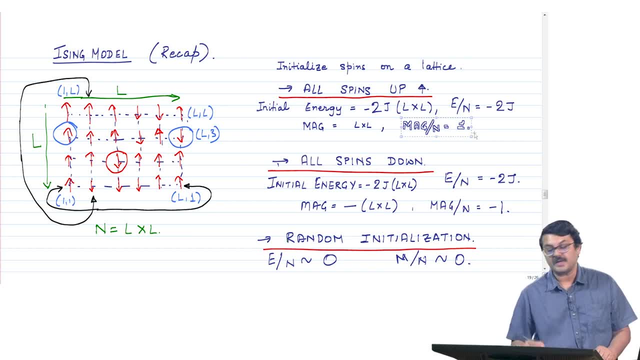 are pointing up. So magnetization per spin is plus 1. magnetization is simply the sum of all the spins in the lattice, the value of the spins in the lattice. If you have all the spins down then the initial energy again will be 2 j into L cross L because 2 spins pointing up or 2 spins pointing down. they 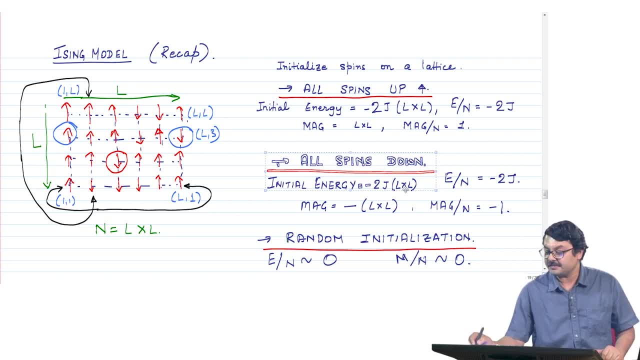 have the same value of the energy, The energy per spin again will be minus 2 j, just as here, but the magnetization for spin, however, will be minus 1.. So if you get these values right, then at least your calculation of the energies is going right. So when, basically, 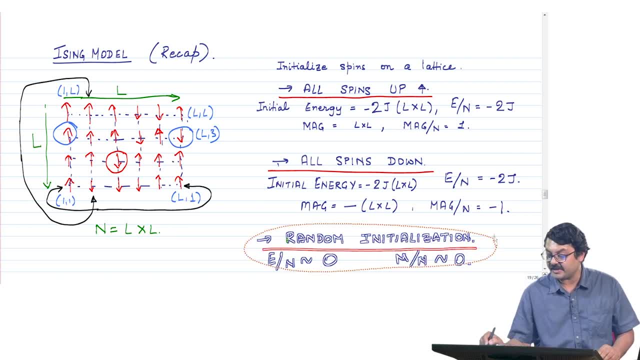 So this is a quick check. However, you can also start with random initial condition and then the initial energy. So half of the spins are pointing up, half of the spins are pointing down. on an average, any spin will have two neighbors which are pointing up two neighbors. 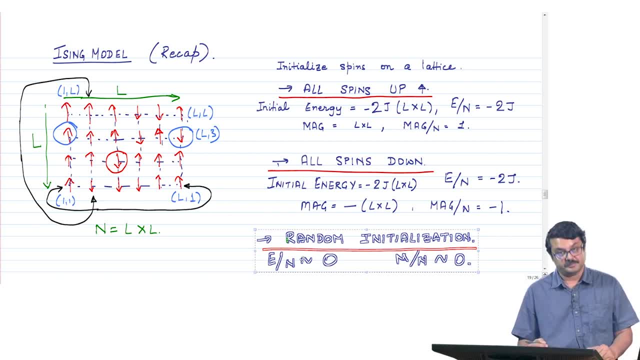 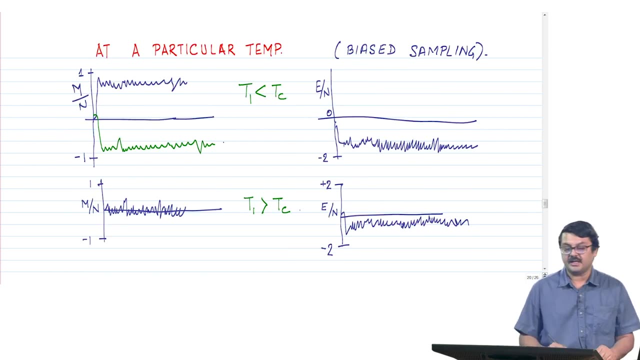 which are pointing down. In that case, the energy per site, the energy per spin would be some number close to 0, it will not be exactly 0 and the magnetization will again also be some number close to 0. ok, Then, what we did in the last class is perform. 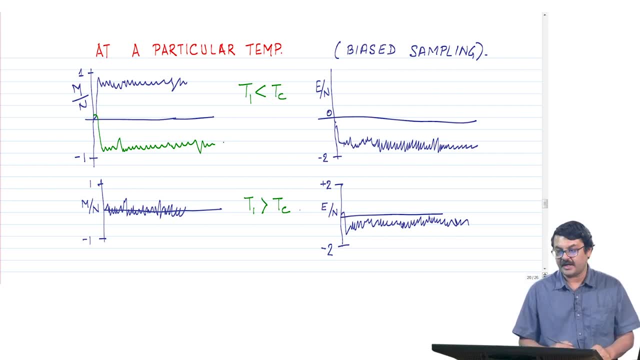 Monte Carlo simulations using the metropolis algorithm. Basically, what we are doing is calculating a spin flip, having a trial spin flip, calculating the energy of the lattice before and after the spin flip. and if the spin flip decreases the energy of the lattice then you accept the spin flip. the magnetization changes and this is a bias sampling. 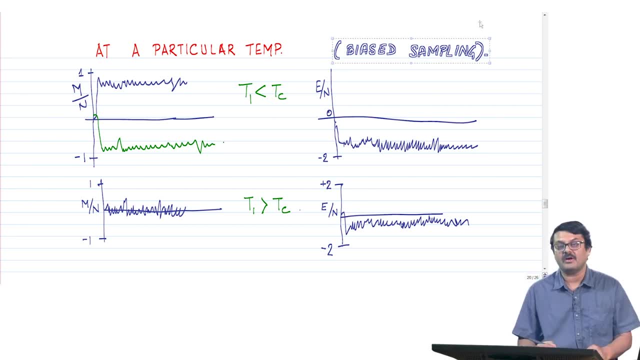 The metropolis algorithm is a bias sampling because any higher energy microstate is accessed with the probability e to the power, delta, E by k, B, T or rather flip due to the spin flip. If the microstate has a higher energy as a consequence of the spin flip, then that 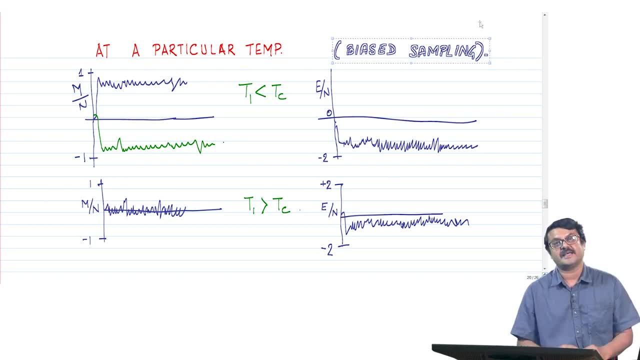 that microstate or that attempt is accepted with probability e to the power minus delta E by k, B, T, right. So what we did in the last class is also plot the magnetization versus number of Monte Carlo steps, and it was fluctuating about a certain value, some value close to. 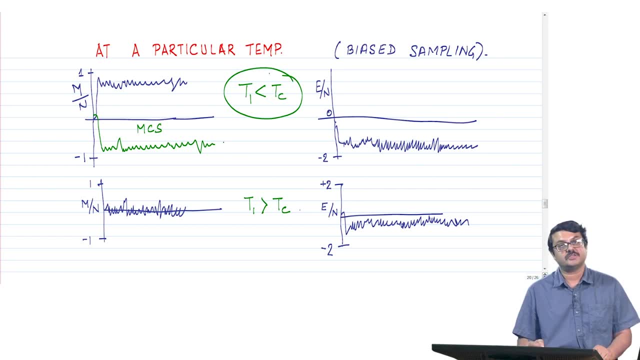 plus 1.. So the temperature of the system was less than T c, the critical temperature, and if you are starting from a random initial condition, initial magnetization would be 0, but it would go up and fluctuate about some average value. Also, if you had a different sequence of random, 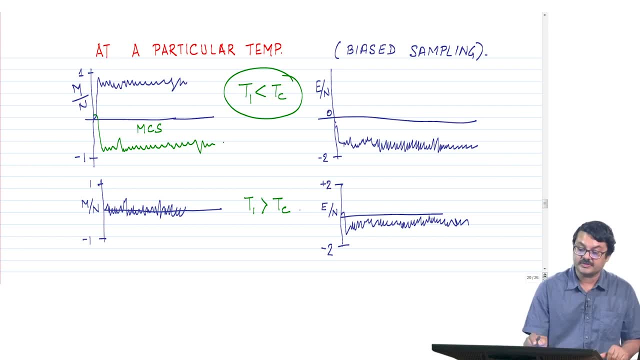 number seeds. it is also possible that the magnetization goes down and fluctuates to a value close to minus 1.. Because all spins, are nearly all spins pointing up and nearly all spins pointing down, have an equal value of the energy. So so both the microstates, which are all spins pointing, 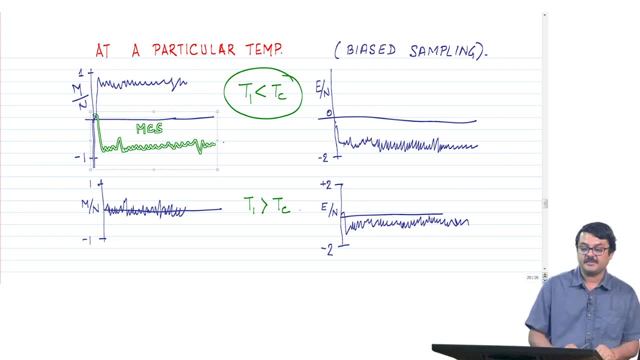 up or all spins, or nearly all spins pointing down, have the same probability right. The energy would fluctuate around just some value above minus 2. if you are in a magnetized state that is T 1 is less than T c, Ok. However, if you chose temperatures which are higher than T c, then the magnetization fluctuates. 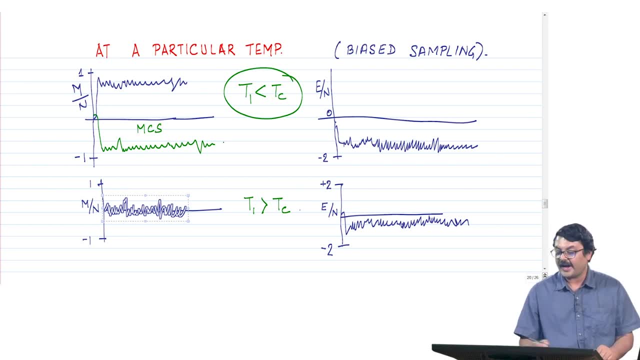 about 0, right, that is what we saw. and the energy, the value of the energy also of the system, also goes to a higher value than minus 2, right, it also fluctuates to about some value close to 0.. So when I am plotting this energy and the magnetization, of course I am talking about. 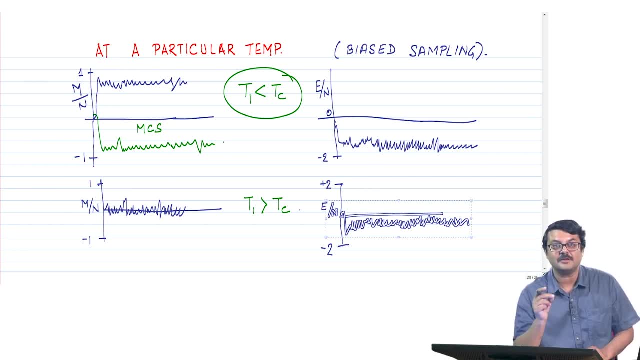 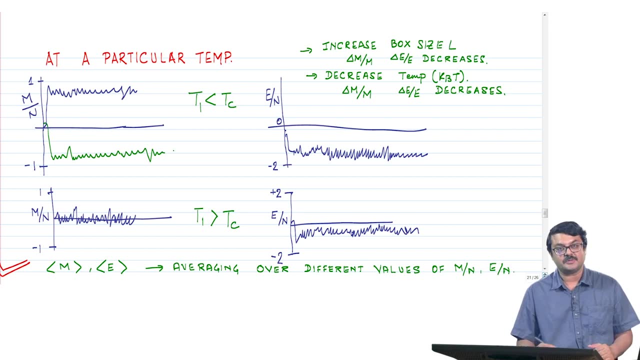 instantaneous magnetization, the magnetization of a particular microstate, not the thermodynamic magnetization, but that the thermodynamic magnetization with statistical physics deals with is basically the average magnetization over all these different microstates, right? So basically M and E. So average magnetization of the average energy can be calculated by. 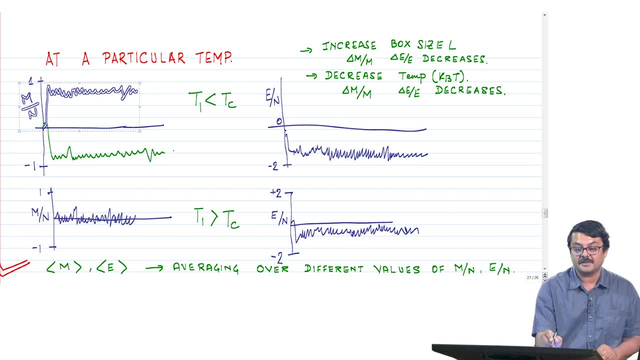 basically taking the values, So the values of these magnetization, of instantaneous magnetization at each of these microstates, and averaging them over. So basically you have magnetization, the instantaneous value of M at after one Monte Carlo step, after the second Monte Carlo step, after the third Monte Carlo step, and just average them over. 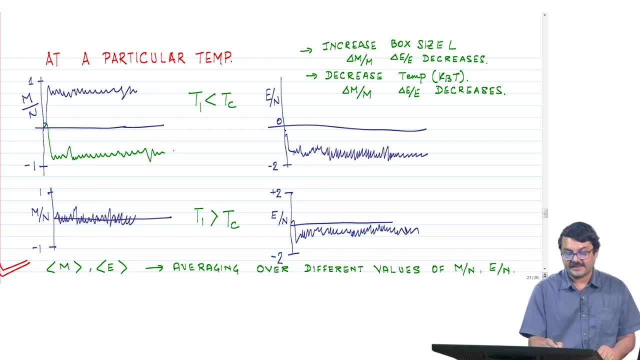 a large number of Monte Carlo steps and then you have the average magnetization E, n. Ok, So that is the principle, but of course, just reminding you, the system will have a relaxation time. So if you are starting from the initial condition, you should first allow the system to equilibrate. 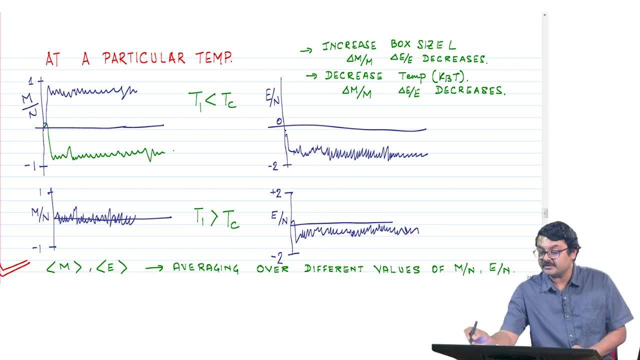 and then start calculating these quantities. We also saw that if we increase the box size, then the fluctuation in the magnetization or the fluctuation in the energy decreases. You have larger number of spins, Hence the fluctuation decreases. Furthermore, if you decrease temperature, right, then also the fluctuation in the magnetization 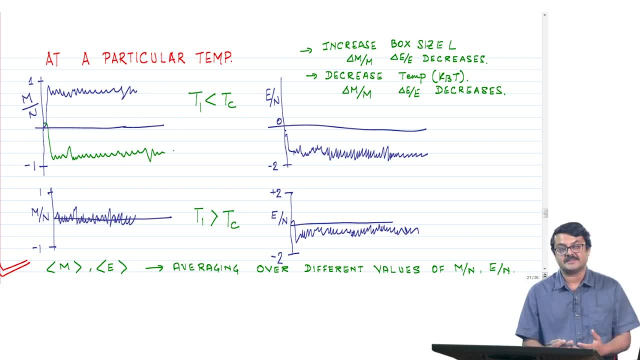 and fluctuation in the energy decreases. that is what temperature does. Temperature basically gives fluctuations to the energy, hence to the magnetization. So if you remember your canonical ensemble statistical physics, you basically: the system takes energy from a external heat path Or gives energy to the external heat path, as a consequence of which the system access. 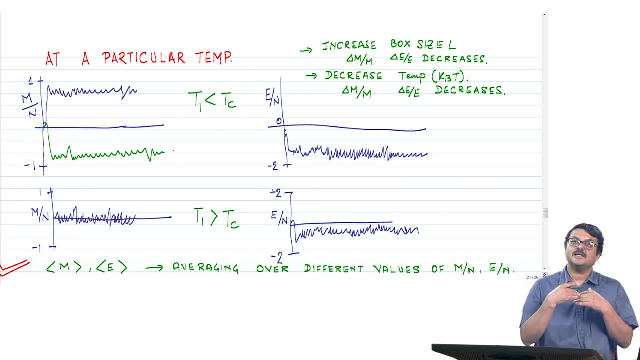 is able to access different microstates of different energies. and that is exactly what we are doing in our Monte Carlo simulation of the Ising model, except we do not have an explicit heat path. I mean, we are not modeled it explicitly, but we are taking in energy. 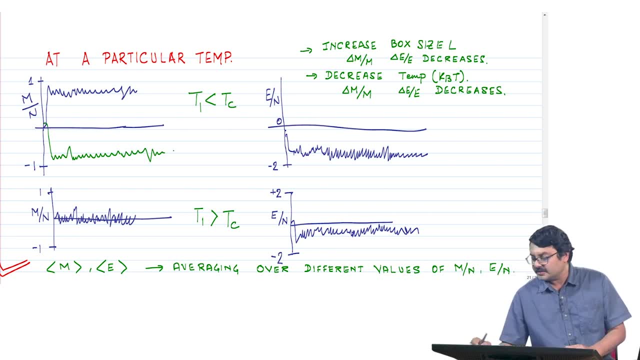 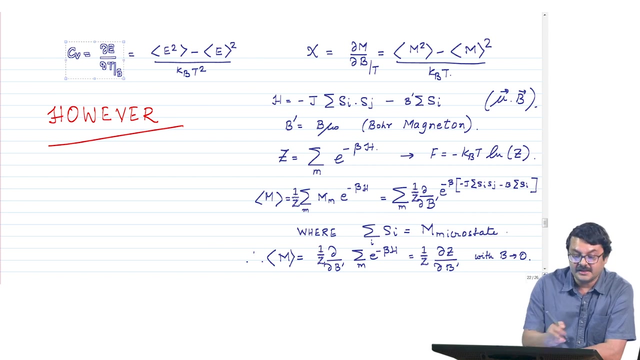 We are giving out energy right. So that seems quite simple. Ok, So you can now have access to those so called thermodynamic quantities, and that is why what the phasist or the experimentalist is interested in. And one can also calculate the specific heat capacity, which is del E, by del t at a constant. 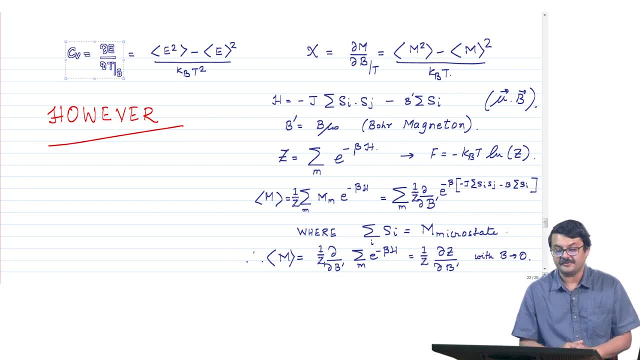 beam and no magnetic field, say, or a constant magnetic field. And you can see in statistical physics- and I think I discussed in one of the previous classes That C, v, Which is del, E, del t, the amount of change in energy of the system due to a change in. 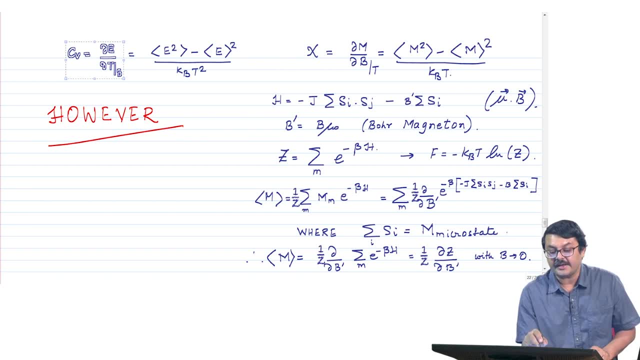 temperature is related to E square average, which is the average energy of the system, not per particle of the entire system. E square average minus E average square, which is nothing but the variance. It is nothing but the variance of energy divided by k, B, T square right, and you can just look. 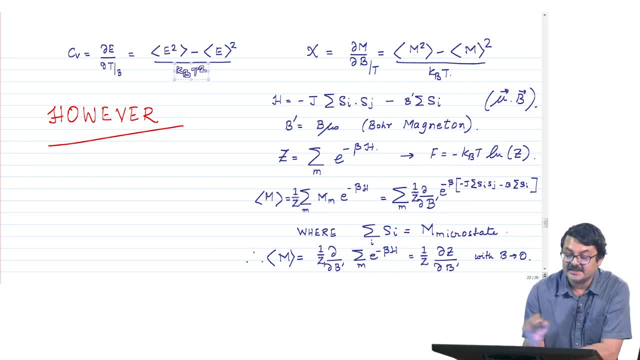 that up. So basically, the specific heat is related to the fluctuation in energy divided by k, B, T square and you can see that the dimensions del E, del t, So it has dimensions of energy per temperature and here you have dimensions of E square energy. 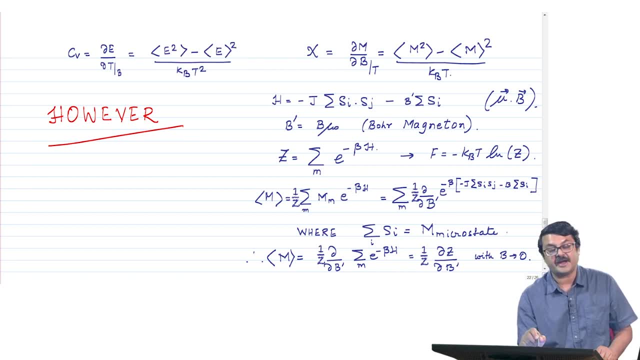 square and you divide by k, B, T, that is dimensions of energy, and then there is an extra t, So the dimensions match, Ok, Ok. So if you calculate C, v, just like you calculate the value of this quantity: E square average minus E average square. 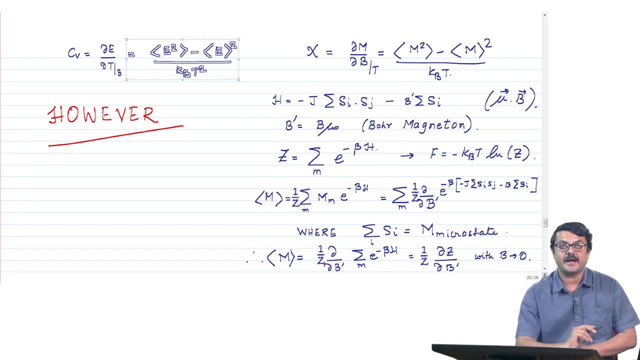 So this, these, basically these angular arrows are, of course, by calculating the value of E square at different microstates as you go on doing the Monte Carlo simulations, at the end of every Monte Carlo step, So you can calculate the value of E square right and then take an average E average. you. 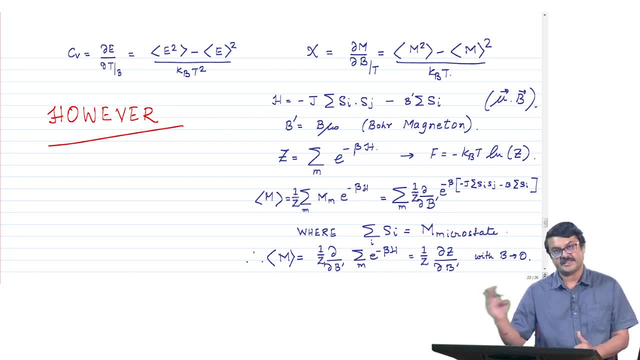 can of course take. when you can calculate the total average, you have basically average the energy over the entire number of Monte Carlo simulations. then you get C v. Similarly, you can calculate susceptibility, chi, which is nothing but del m, del B. del m means when you switch on a magnetic field. 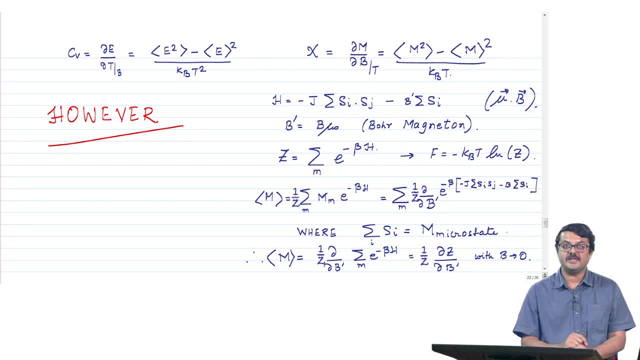 And so there is a slight difference. Ok, So there is a slight perturbation in the magnetic field. B, then how much is the change in magnetization? that is what the susceptibility chi measures, And one can check that. basically, chi is related to m square average minus n average square. 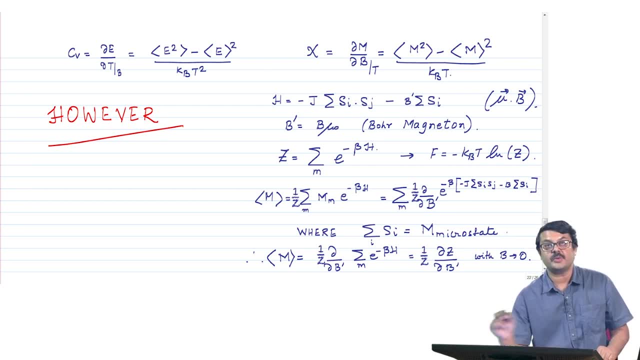 by k, B, T. So m square average minus n average square is nothing but the variance in magnetization, right? So this is the variance expression for the variance. One point till now, when we wrote down the Ising Hamiltonian, there was no B, though no. 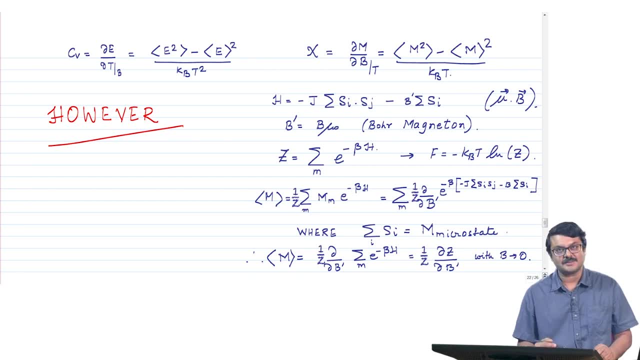 magnetic field B, right, So where does susceptibility come in? So, basically, and how can you calculate susceptibility m? by using the variance. just to give you an idea. and So the Hamiltonian H was minus j m. So this is the variance expression for the variance. 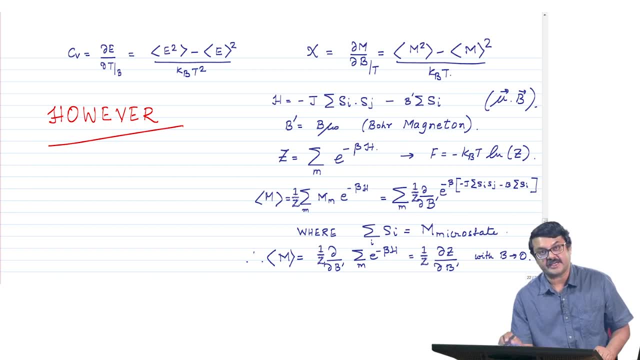 So, basically, and how can you calculate susceptibility m? by using the variance, just to give you an idea, and So you can write it down: minus j, SI, dot, sj, sum over all spins. right, and you can also add a term which is nothing but minus mu, dot, B, mu being the magnetic moment of each spin. 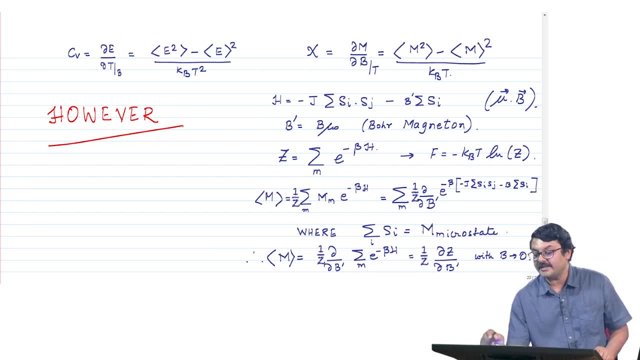 into B, B being the magnetic field, And here, since we are writing in terms of essentially the spin, where basically mu is nothing but the Bohr magnet, Right magneton, into the spin. So hence I have written, instead of magnetic field, I have written at: 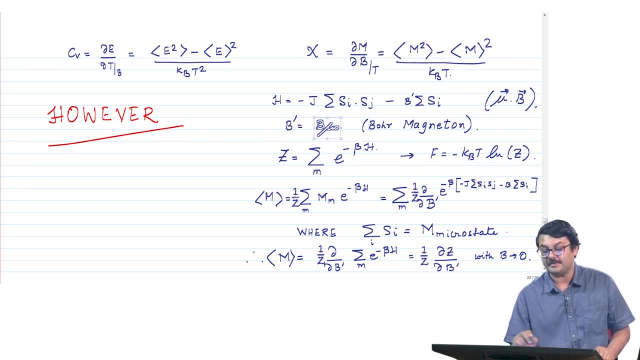 B dash, where B dash is nothing but the magnetic field, B into the Bohr magneton. So you can also write it like this: and then in this case the partition function z will be e to the power minus beta s sum over all possible microstates. the free energy is of course minus k bit. 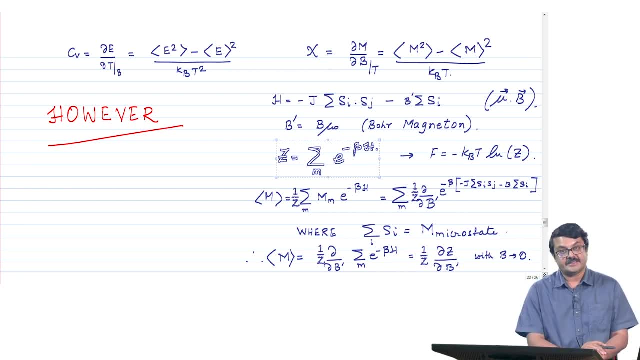 ln of z and the average magnetization. right can be written as the m subscript: small m, which means basically the instantaneous magnetization. the magnetization at each microstate. the average magnetization is basically sum over all possible accessible microstates, the magnetization. 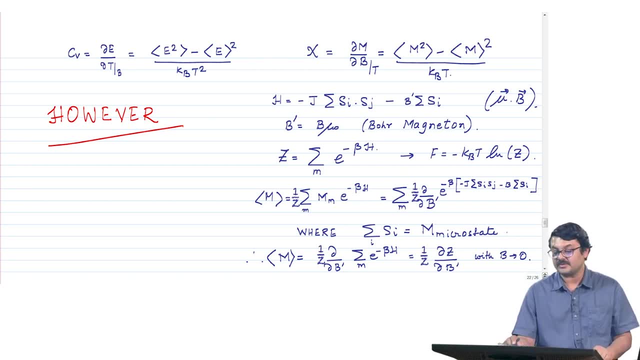 of that microstate, the instantaneous magnetization of that microstate into e to the power minus beta Hamiltonian energy right, And this can be written as basically as sum over all microstates here minus del del B dash, B dash being the magnetic field expressed in terms of Bohr magneton. 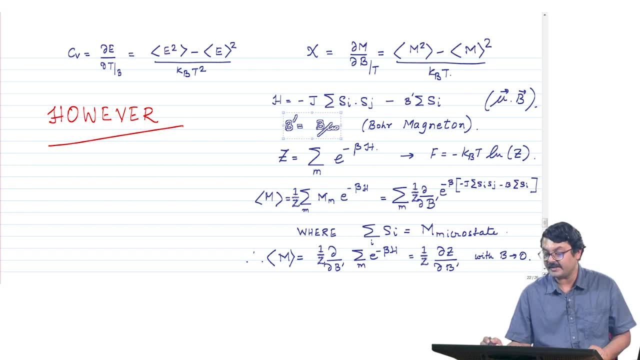 So this rescaled magnetic field del del B dash into minus e, to the power minus beta, beta 1 by k B, T minus J, i, minus J s, i bar i dot sj. summation minus b dash, summation s i right. So basically where, if you take? 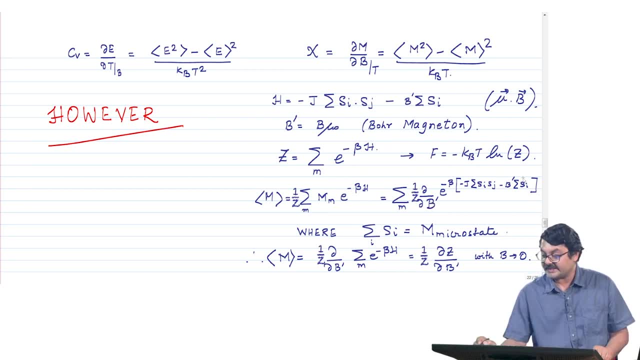 a derivative with respect to b dash. basically, this sum of s? i will come down in the denominator right. this is an exponential function, And sum over s? i, the total sum of all the spins in the lattice, is nothing but the magnetization of that microstate right. So basically then, 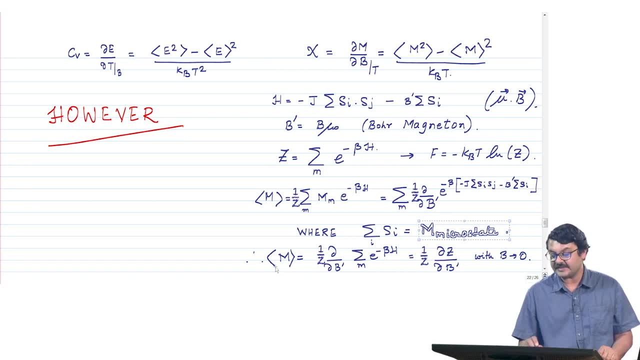 the average magnetization in statistical physics can be written as minus del del b dash into z, which is derivative of the partition function with respect to b dash or the magnetic field, and later we can take: b tends to 0, right. So hence what is the point? The point is: 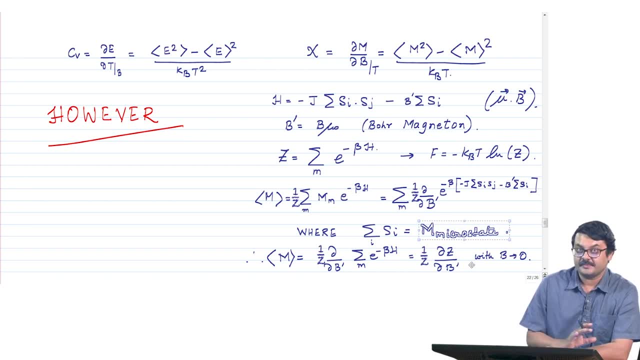 basically, even though you do not have an explicit magnetic field in the system or you are not modeling that explicitly when we wrote our code, You can get the chi susceptibility right even in the absence of magnetic field, calculating it from equilibrium properties. right is related to the m square. You can just check that if. 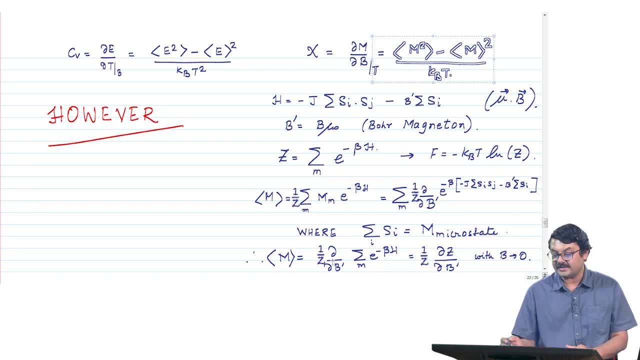 m square minus m average square, it will be nothing but double del m del b. you can carry this step out for once more right? You take the derivative of this quantity with respect to b and you can get m square minus m average square by k, B, T, because you will. 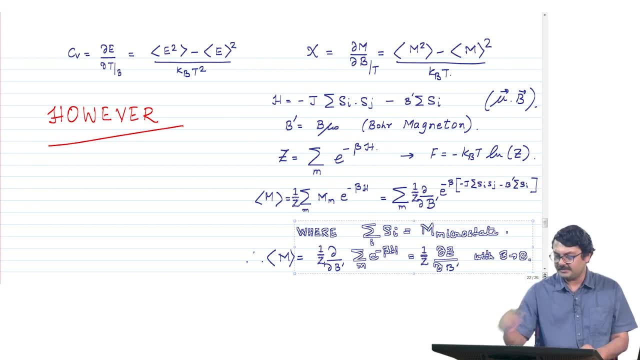 also have a beta factor there, right, and the beta will also come down, which I have not written here, but you can fill that in, ok, So that is it. So on principle. basically, if you are able to generate different microstates, then you. 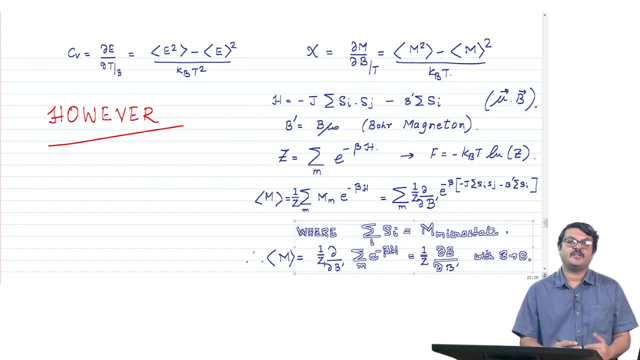 can calculate m average, m average, e, C, v, chi, over these different microstates which we generate in our computer, and we can compute all the properties of the system. We can also basically calculate these quantities as a function of temperature, So you can basically study the phase diagram of the system, However. however, before you, 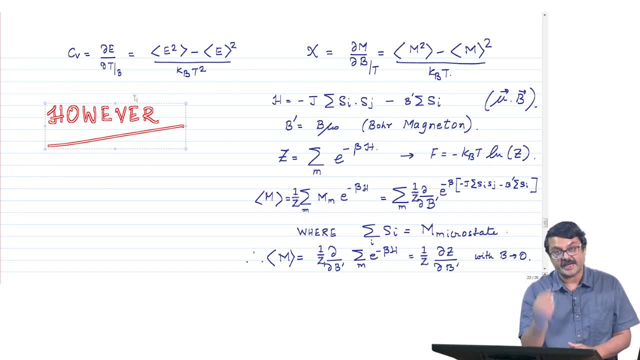 complete. however, before you start calculating these things, there are some other issues or artifacts of simulations to be aware of, and only after fully understanding those issues should one start calculating the average magnetization, the average C, v, chi, and so on, so forth. 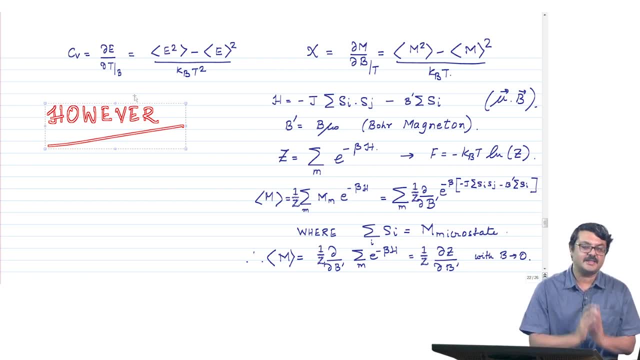 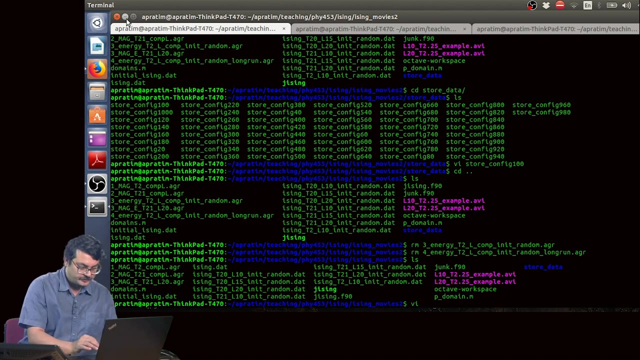 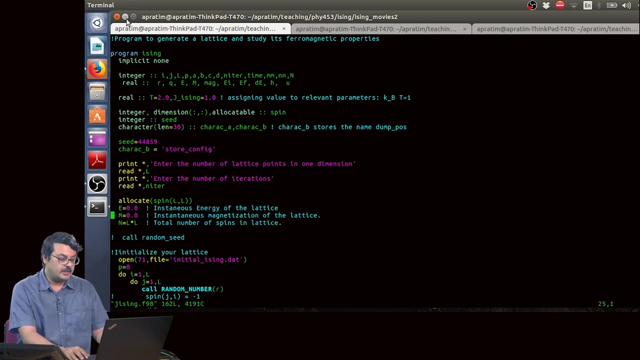 the computer and see the data, and let us learn a bit more about the artifacts before coming back to the physics and calculating C, v, chi, m as a function of temperature. ok, So looking at the code again: v, i, j Ising dot F90, what we want to do right now is basically: 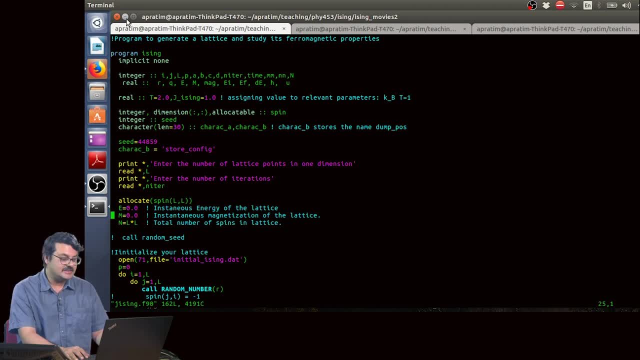 plot: magnetization energy versus Monte Carlo step MCS for slightly smaller box sizes. So we already did it for box size 40 and 60 and 80 in the last time and we saw all the energy fluctuations. but if we have slightly smaller box sizes- box of 10,, 15,, 20- let us see if. 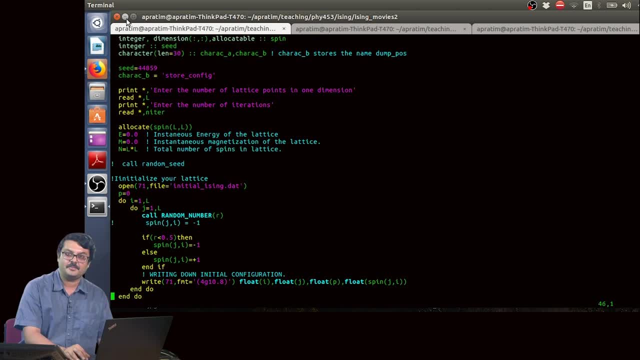 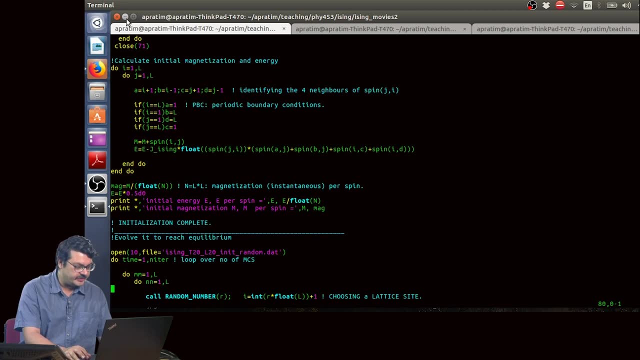 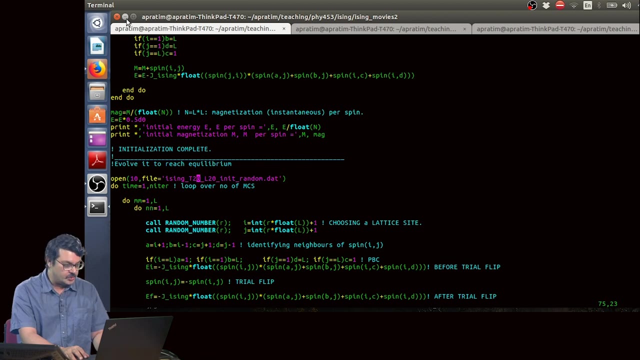 we see something strange or unexpected when we plot the magnetization energy Versus MCS. ok, So all that I am doing here is basically I am going to run the data at temperature T equal to 2, box size equal to 20,, right, and all the data, which is basically. 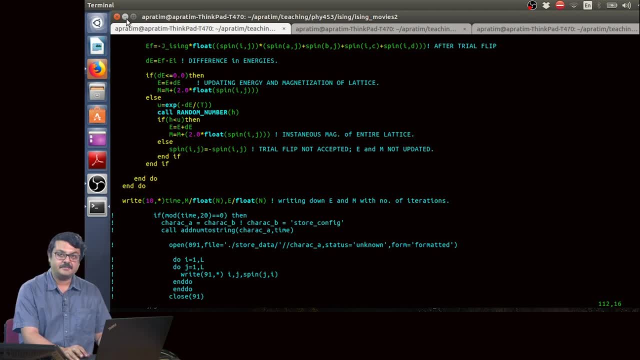 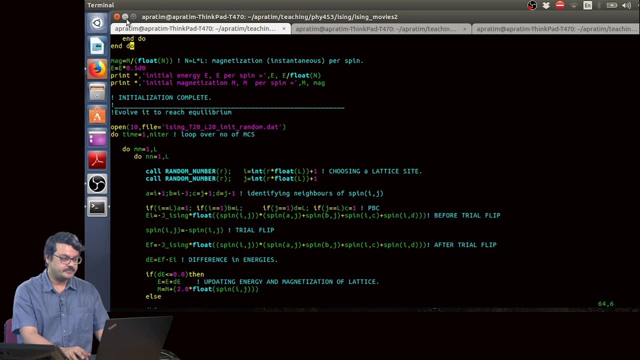 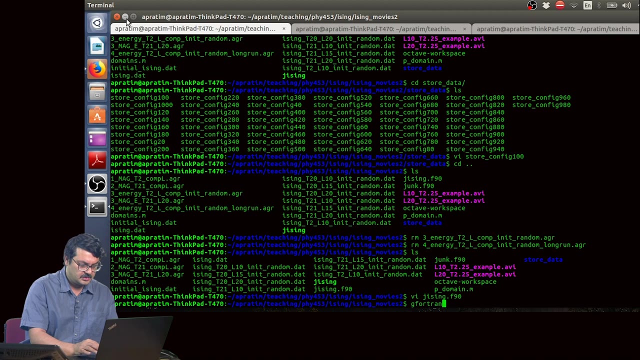 the time. here is the time. the magnetization per spin and the energy per spin is going to be written down in this Ok File, just as previous times. right, So g Fortran minus O, 3 j Ising dot. F90 minus O. 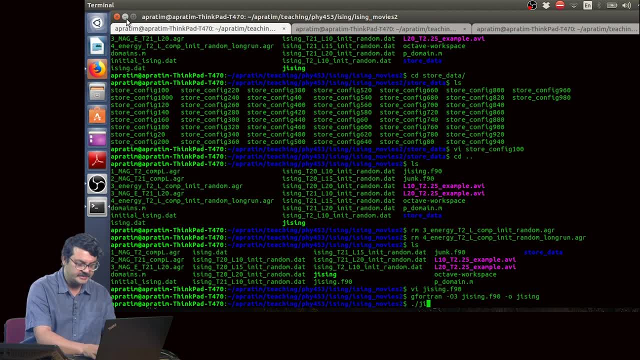 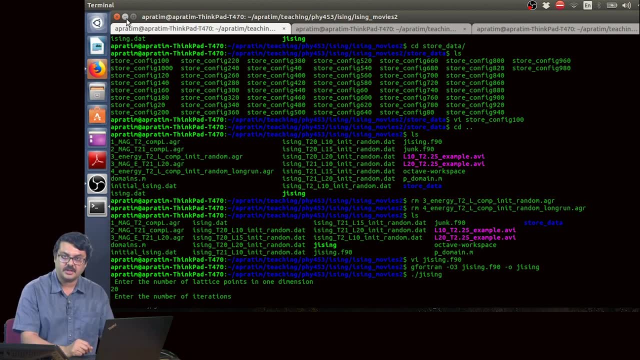 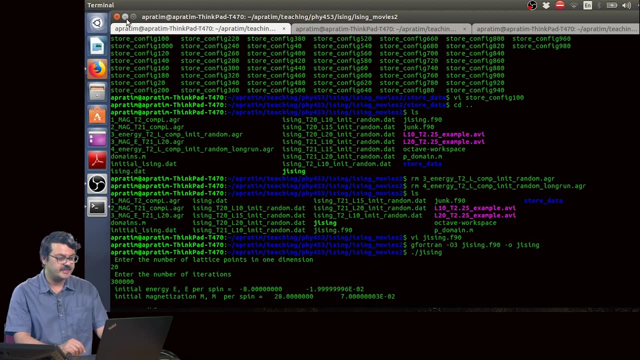 j Ising compile and j Ising. I am going to run the code 20, the temperature is already given as 2 in the code, just as we did it last time, And of course we have 3,00,000 iterations. 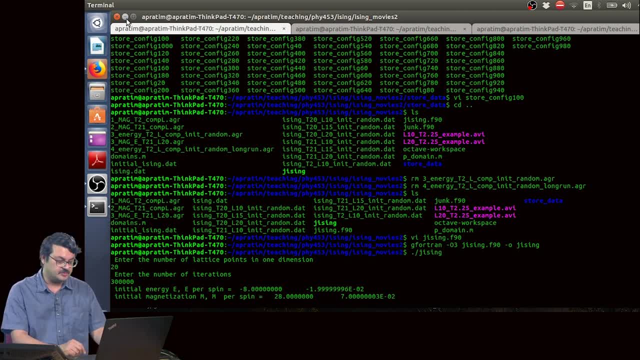 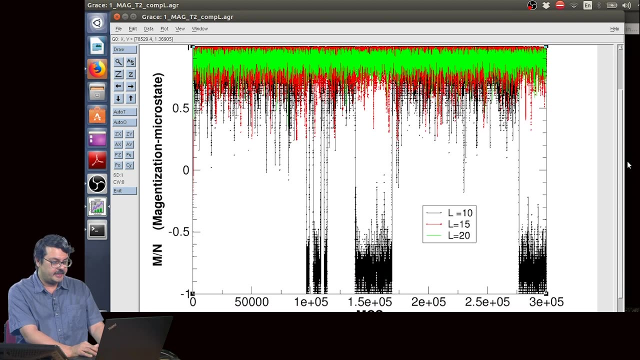 Now I have already done the simulations for different box sizes and what I shall do is basically just show you the data. I have plotted it. so this 2D Ising model, And basically I am plotting magnetization per spin versus MCS, the Monte Carlo step, and I have showed above It is the U-shaped number. So mc 1 is together per unit, Then mc 2 is omega and omega is also equal to omega. Then I am making some random calculations for those problems, So that basically that was everything To summarize the pattern we were having just now. What is the graph number? well, the hetero bright resistance is. we did a basicμ of yesterdays, just like that Next one. you cannot do that. So who is going to write disturbed densityogram? then a perfect: how many membkle we are going to write down. I am gonna. 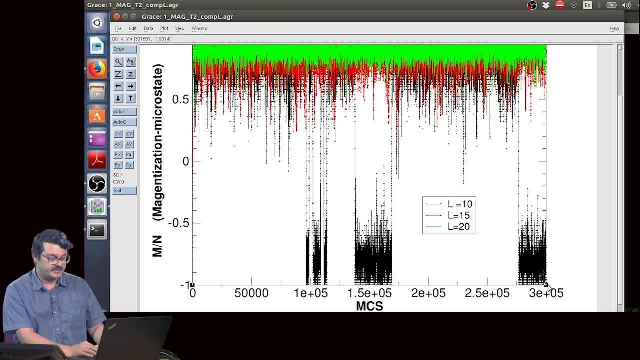 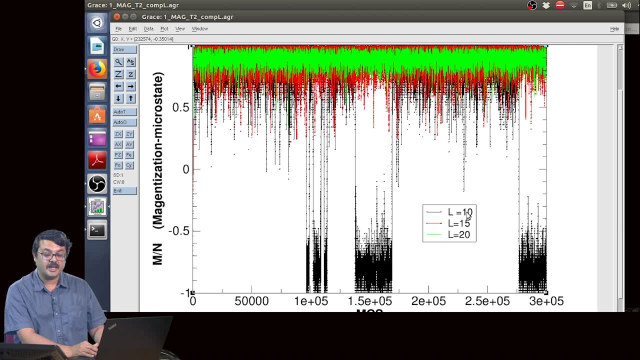 showing the data for 3 lakh iterations right Now. the black data is for L, the lattice size equal to L, equal to 10.. So you have 100 spins in the lattice. the red data is for L, equal to 15, and the green one is for 20.. Now there is something which you did not see last time. 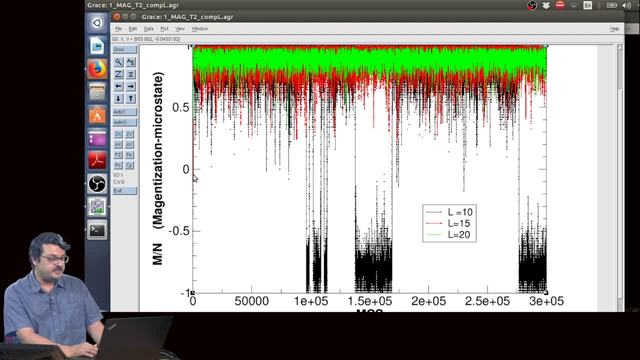 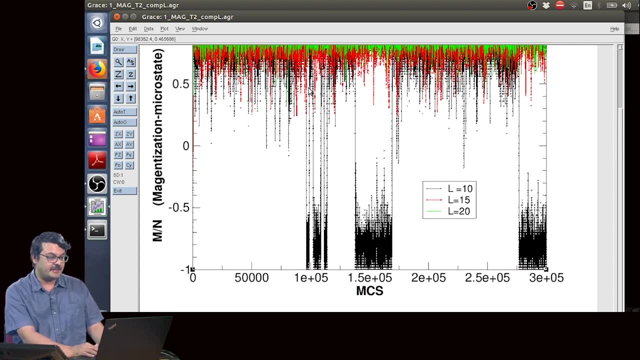 when you have L equal to 10, starting from a random initial condition, the spin, the magnetization, the instantaneous magnetization essentially went up some number close to plus 1, ok, But after fluctuating for some time you see that the magnetization has gone from some. 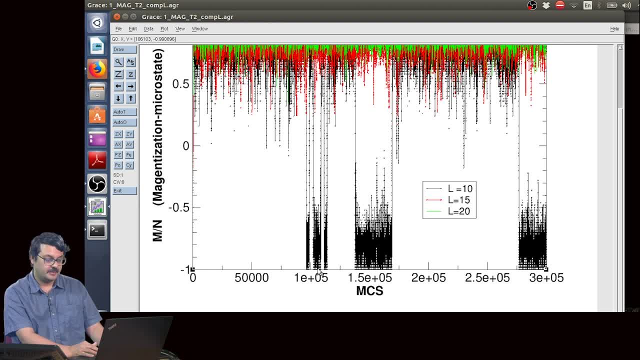 number close to plus 1, to minus 1, and then here it goes up again and comes down again, and here there is a gap and here again it goes up to plus 1 and here again it fluctuates about minus 1.. Of course, the average energy in these two states either close to plus 1 or minus 1 is. 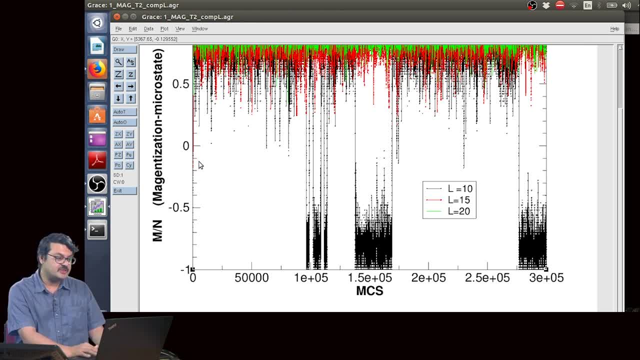 the same right. So. but previously we saw that the energy was going up or down and sticking and fluctuating about some average value. but here we see that the state of the system is going from plus m to minus m. Now, if you just took an average for L cross for L equal. 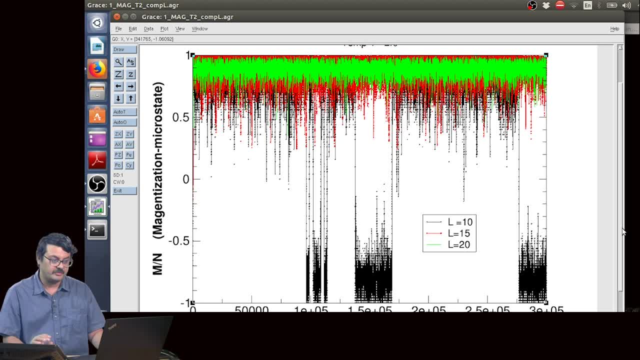 to 10,. if you average the magnetization over a long run right in the previous cases, you would get a constant value. but here, since sometimes it is plus 1, close to plus 1, and sometimes it is close to minus 1, if you take a good average you will get a 0. So why is? 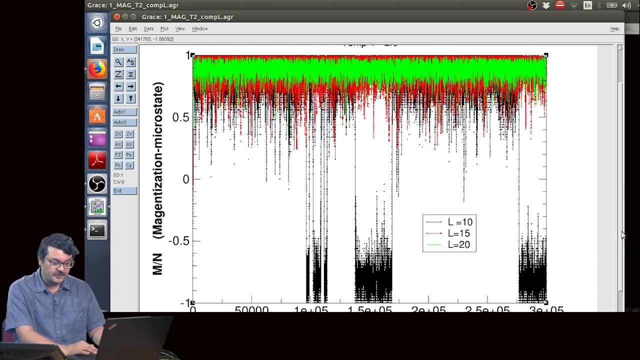 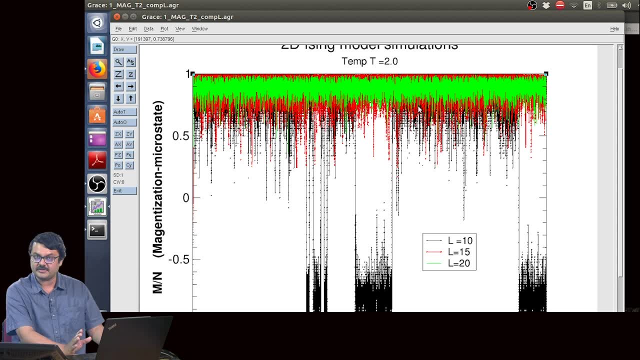 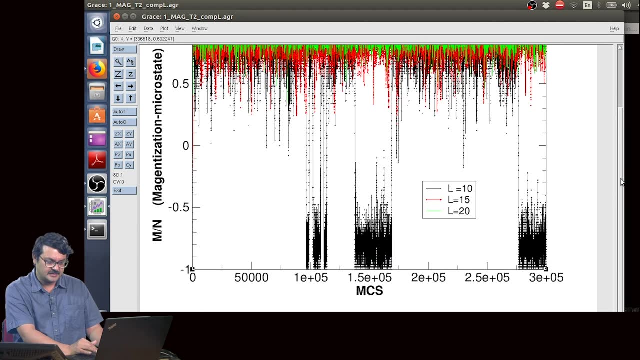 this happening? ok, So this is the question. whereas for larger lattices, L equal to 15 or L equal to 20, you see it is fluctuating about some average value, just as. So this is what we have seen it previously. Now, the L equal to 10 case is a bit strange. 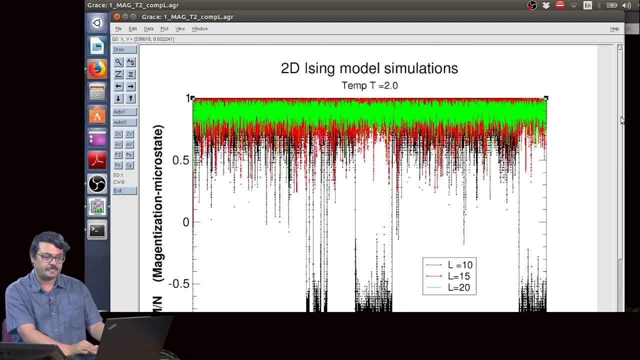 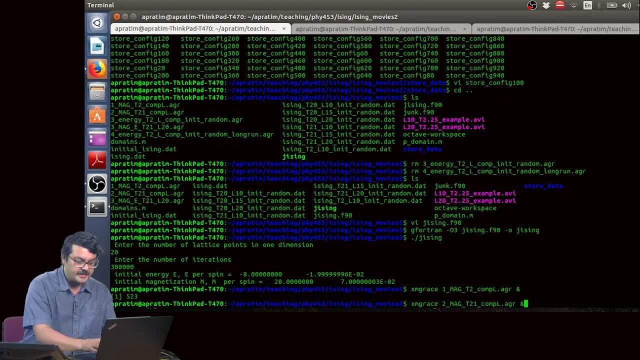 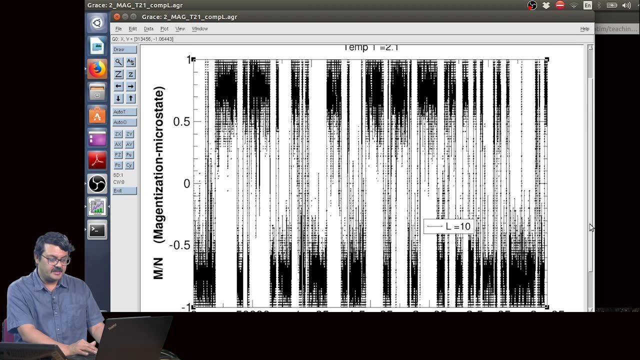 So let us try to see what happens when you increase the temperature slightly. ok, So I have already done that and here is the data for L, equal to 10 up to 3 lakh iterations, ok, Monte Carlo steps equal to 3 lakh, and the number of iterations at temperature of 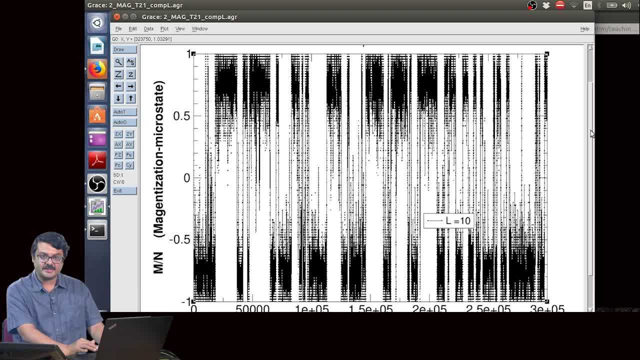 2.1.. And here we see, when we increase the temperature to 2.1, there are rapid flips where the magnetization of the L equal to 10 lattice goes from plus, from plus to minus, back to plus, back to minus, and so on, so forth. it becomes much more frequent. ok, What about L equal to 15 and L equal to 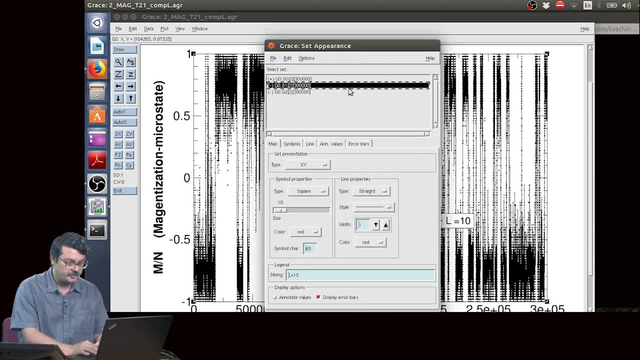 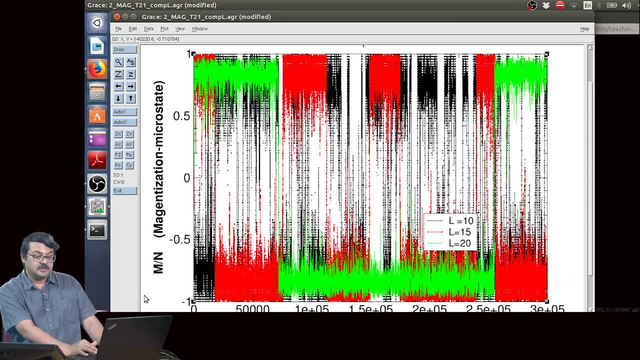 20?. So I have already plotted it, I will just switch it off. Ok, Ok, Ok. So when you go to L equal to 15, again now at a slightly higher temperature, the spin goes from minus 1 to plus 1, again back to minus 1, again to plus 1, but for a higher. 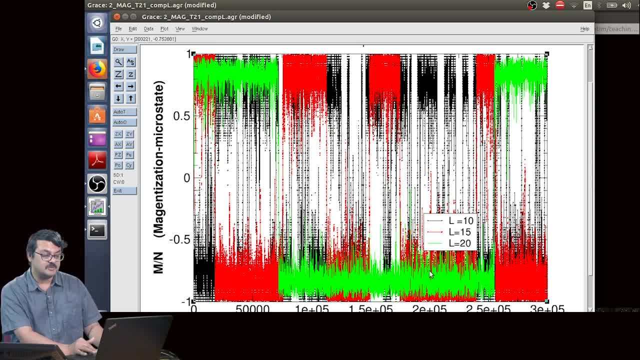 the size of the lattice, this jump from plus 1 to minus 1 becomes less frequent. ok, With the increase in temperature the frequency increased. but as you increase the lattice size, So the jump from plus 1 to minus 1 is less frequent. If you remember, for L equal to 80. 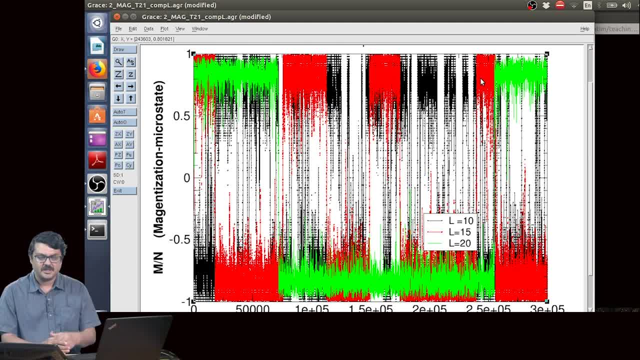 L equal to 60, over 1 lakh iterations. we hardly saw such behavior. Now, this is very odd and fishy, because if you have a magnet, right, So what is this plus 1 to minus 1 mean? basically, the magnetized magnetic state is flipping. So if you, if you take a real magnet, if you 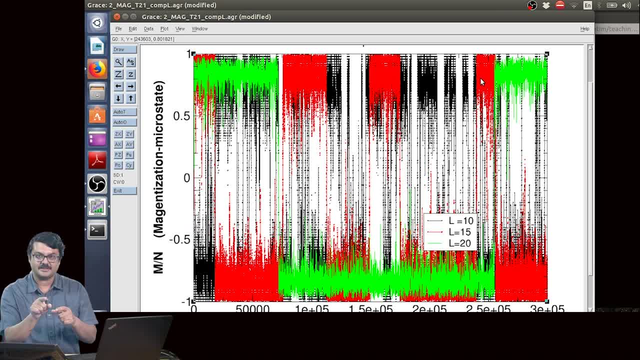 keep it, Ok, Ok. So in this direction in the morning. you do not come back in the evening and say: the see that the North Pole has become in the opposite direction. the North Pole and the South Pole does not flip right. So the magnetic state is it is either plus 1 or minus. 1 is basically. 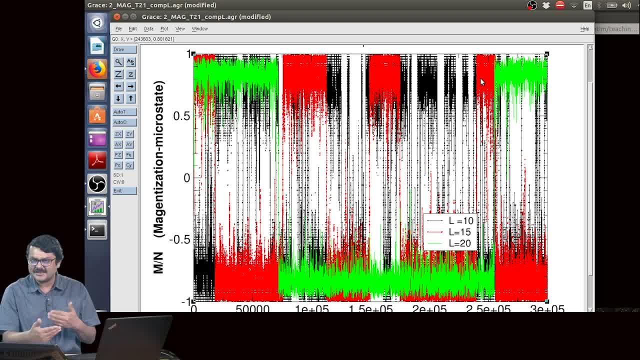 saying that the direction of the magnetization it and it does not flip really. So why is this happening? So this is a finite size artifact. So let us explore this a bit more detail, because unless we understand what is happening here and we take a naive average, we will get 0 magnetization. if we average over all micro. 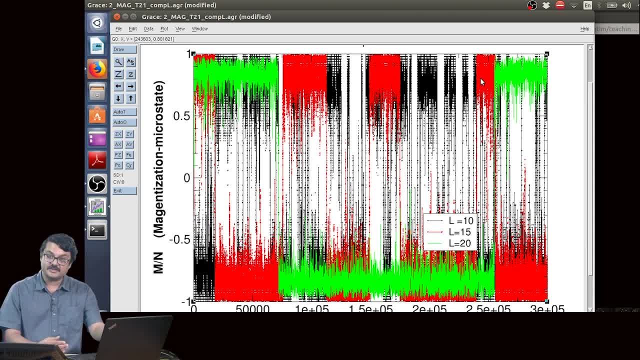 states, especially at temperatures close to T c. when you see such large flips happening and the you will get 0, because half of the time the system is in the plus state, half of the time it is in minus state. Magnetization- the magnetic state is still not. it is not unmagnetized. 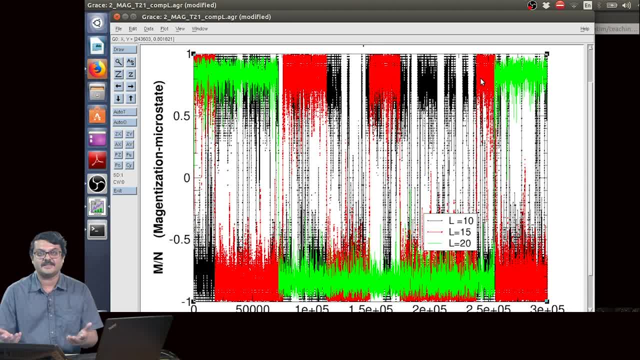 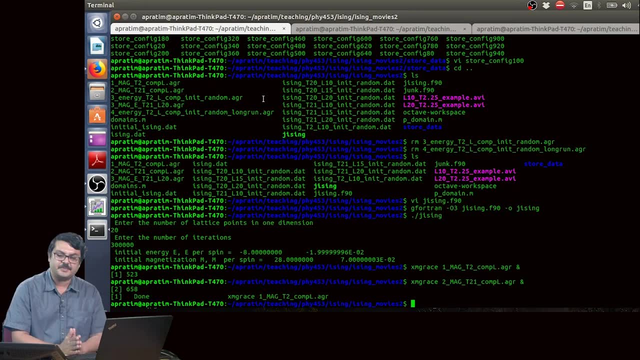 it is either plus 1 or minus 1. if you take the average, you will get a 0, which is an erroneous value. why is this happening and how do we overcome such issues? To understand that, let us look at what the spins are doing more explicitly. ok, So what? 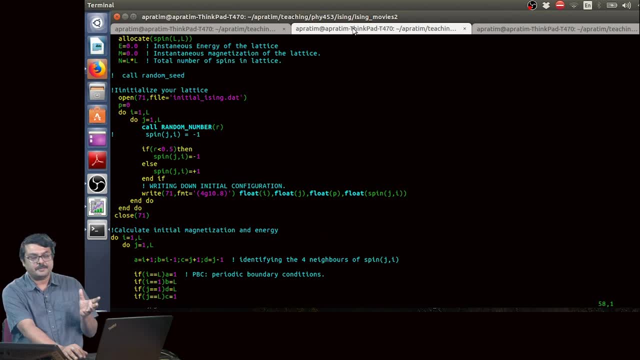 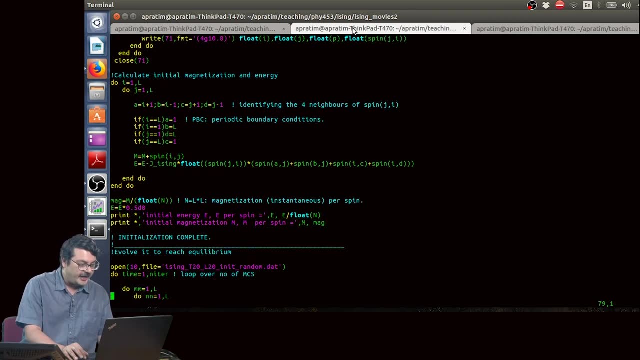 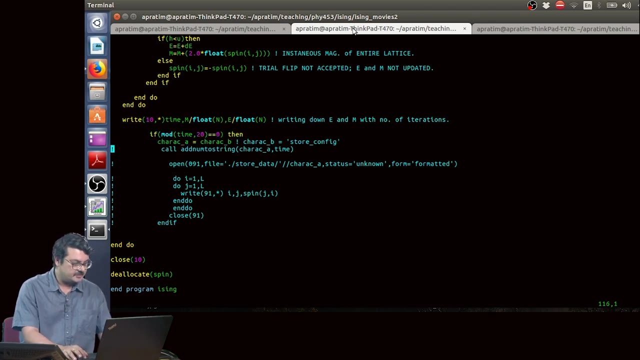 I am going to do is basically show you a movie of where I explicitly follow each spin as a function of time, and the way I do it is basically: I have some commented out statements, I comment them in. So here, all that is being done in these steps. 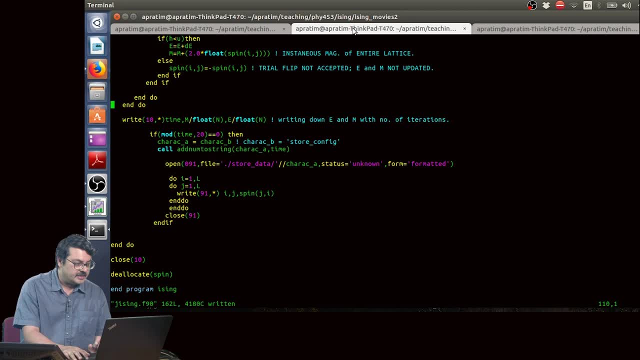 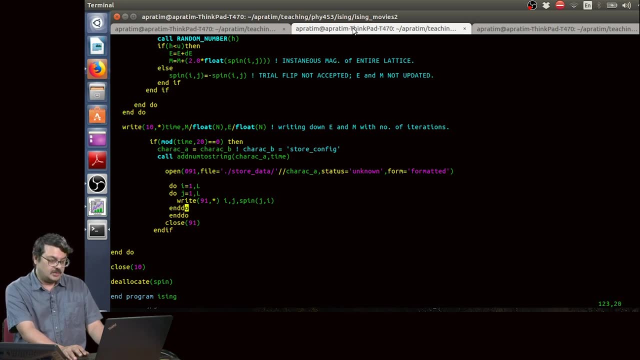 is after every around 20 Monte Carlo steps, I am writing down: i equal to 1 to L, j equal to 1 to L. So I am going to each point in the lattice and writing down the coordinates. i and j are the coordinates of that lattice point and 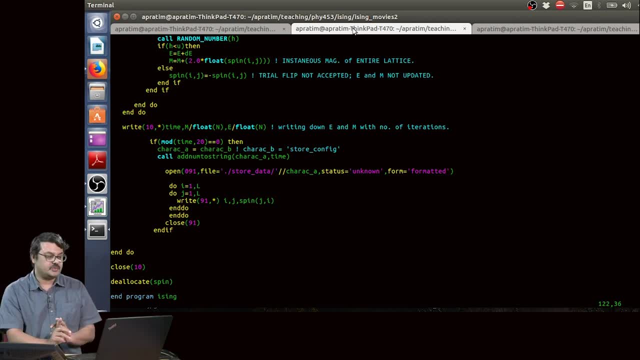 the value of the spin at that lattice point. So what is happening is, after every 20 steps I shall explicitly get to see what is the spin state. right, We are already calculating that, but here we can follow each an individual spin And we write down the spin state. So we are already calculating that, but here we can. 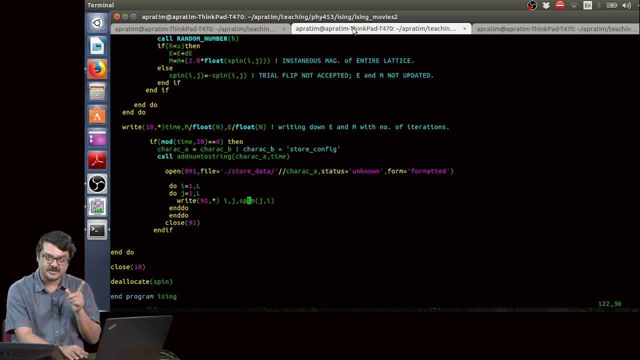 follow each an individual spin and we write down the spin state. So we are already calculating the micro state, the position of each spin in a file, right, and what I am going to do is then make a movie file and see it so that we can follow it. 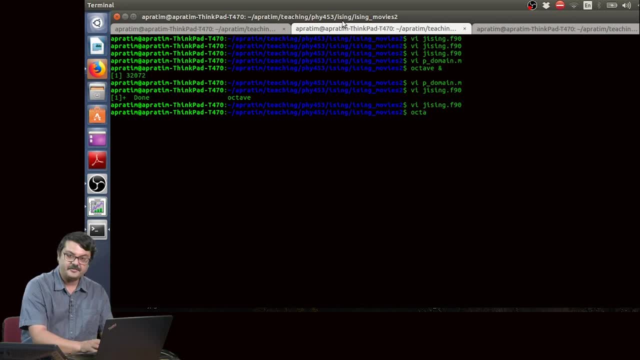 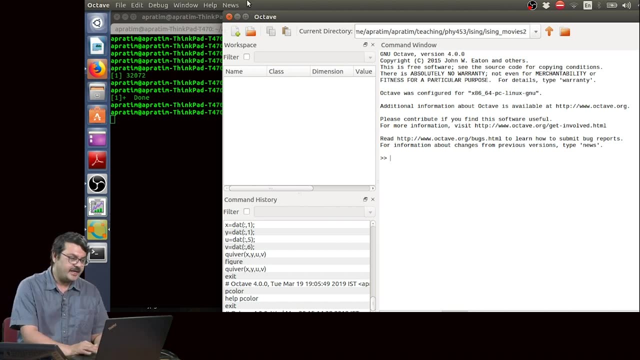 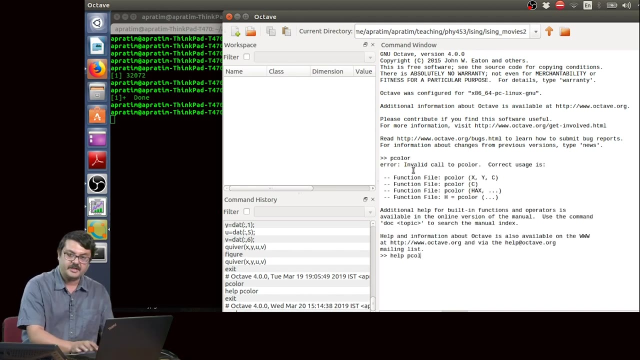 To make the movie file. you can use the software called octave. it is equivalent to the MATLAB, except that octave is free, is freely downloadable, and I am going to use the command called pColor.2, to basically plot all the data. So I have already done that and you can learn this on. 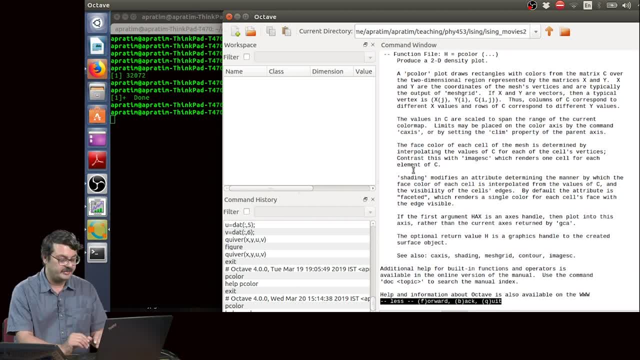 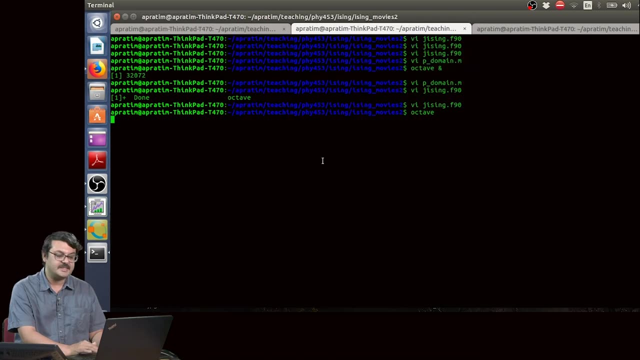 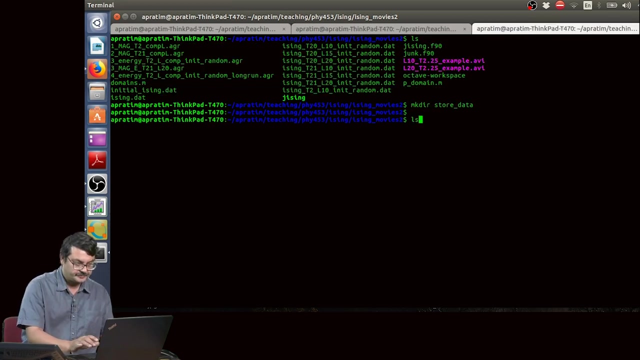 your own, if you want, by reading about p color and reading about octave. but what I am going to focus is I have already saved the positions of all the spins, every 20 iterations, in some file and I am going to basically show you the movie about the state of those spins. 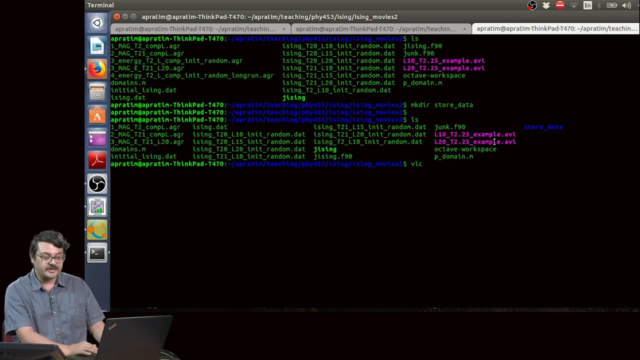 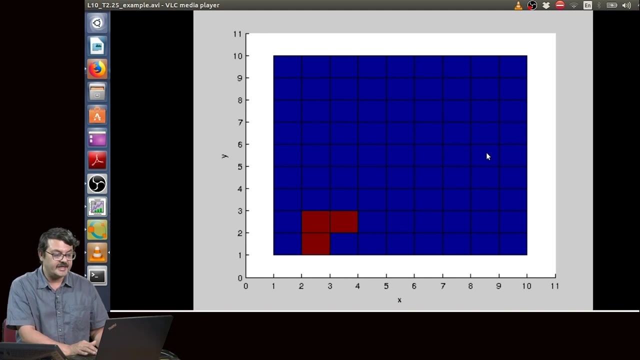 So this is for a 10 cross, 10 lattice at temperature of 2.25 and let us see what happened. So just to stop it, let us suppose here you see, that the entire lattice, blue suppose transform for spins pointing up, red stands for spins pointing down, and at temperature of 2.25 you. 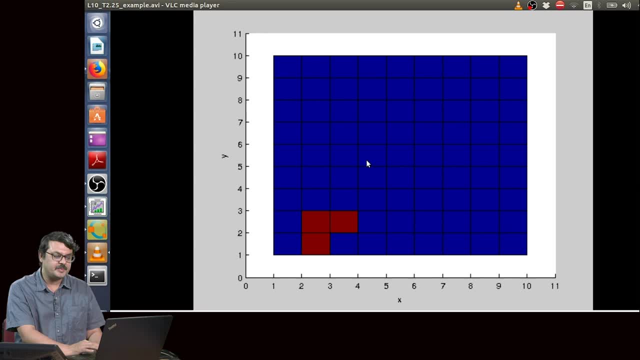 see, most of the spins are pointing up and 3 spins are pointing down. So basically the magnetic state is plus 1, some number very close to plus 1, but as we evolve the system through Monte Carlo steps, you see that there are fluctuations right, and suddenly the entire. 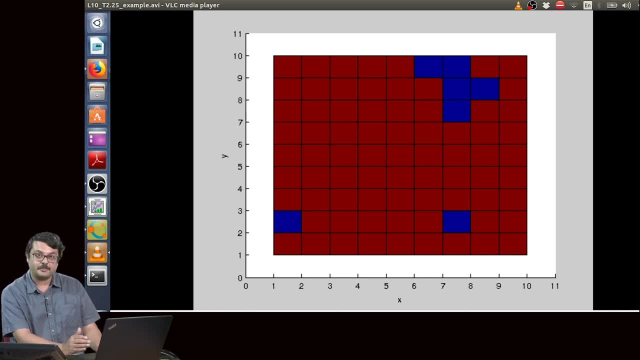 state of the All. the system has changed where all the spins are pointing up. So these are these red colors have basically, sorry, they are pointing down. red was corresponding to spins pointing down in a few. only a few spins are pointing up. So basically, the magnetization has gone from.